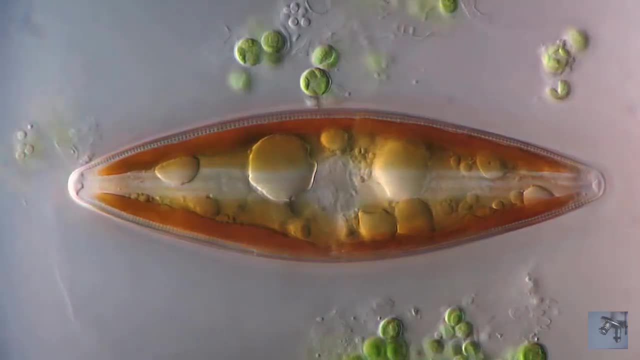 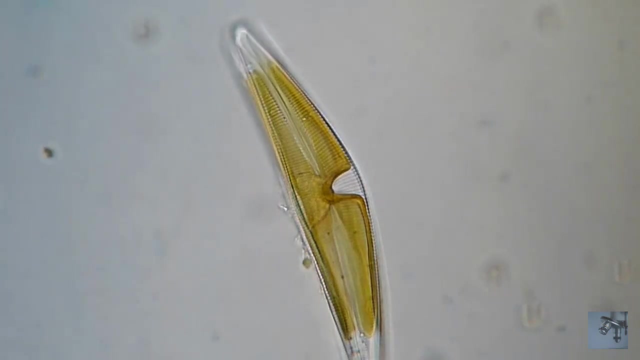 Many diatom species are planktonic, suspended in water, moving at the mercy of its currents. Others remain attached to submerged surfaces. A single diatom cell can divide and form two new cells. Cells may divide as quickly as once a day, up to once every several weeks. 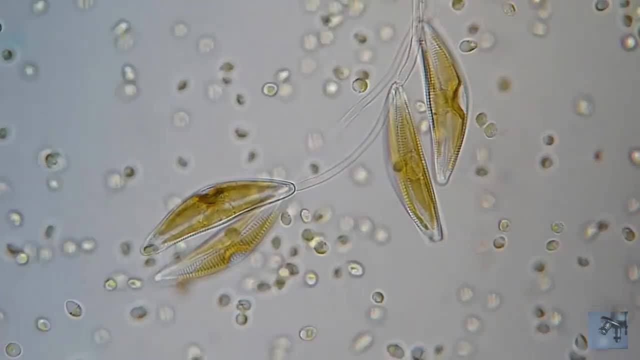 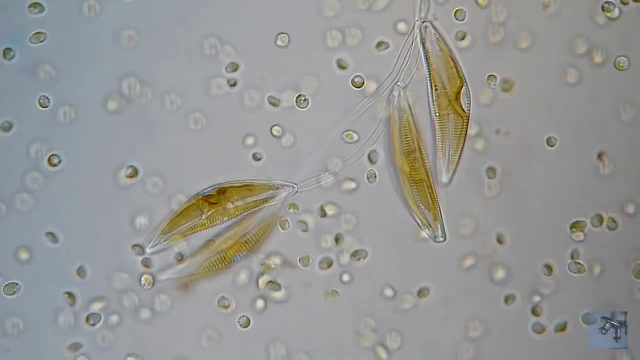 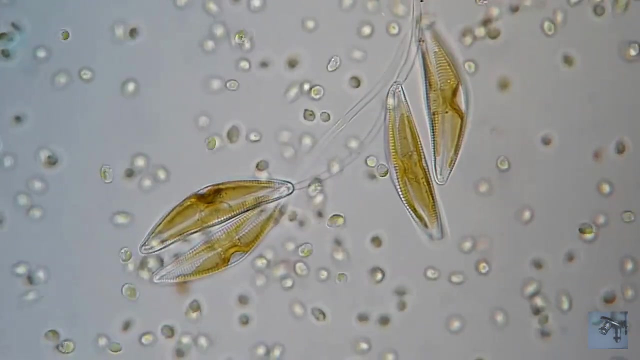 However, the silica cell wall is sort of a biological constraint because with each cell division, diatom cells become progressively smaller. The daughter cell forms a new silica cell wall inside the parent, But the rigid glass cell wall cannot expand. The baby is stuck for its entire life, being smaller than the mom. 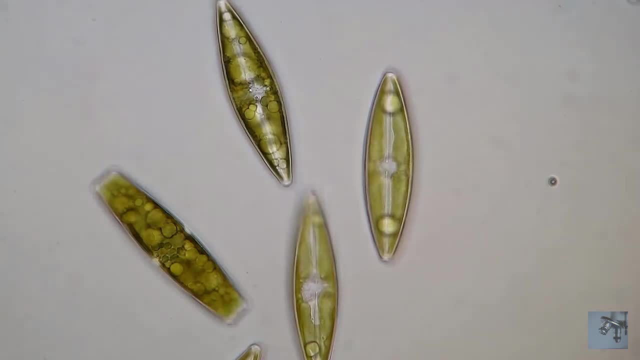 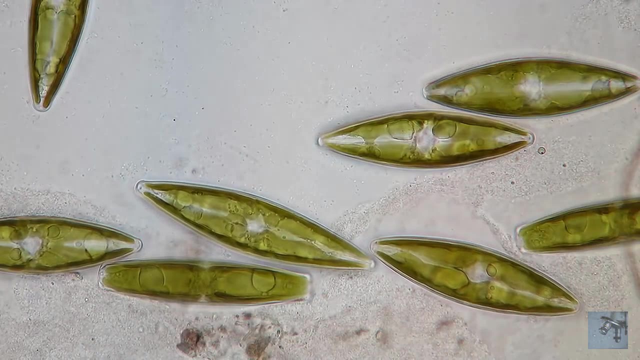 The solution to this problem comes through sexual reproduction Diatoms. regurgitate Diatoms regain their maximum size through sexual reproduction in the formation of a special structure termed an oxospor. Oxospors are unique types of cells that possess silica bands called. 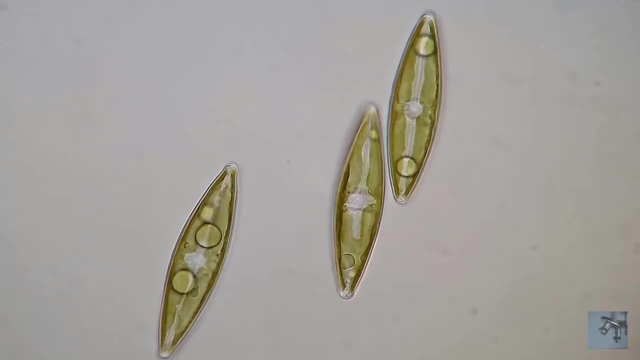 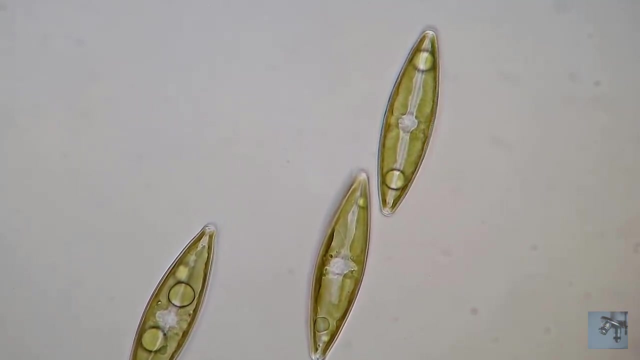 parazonia rather than a rigid silica cell wall. The parazonium allows the cell to expand to be its maximum size. Previously, scientists had observed the complete life cycles in barely a handful of diatom species, And even among well-studied diatoms, sexual reproduction had 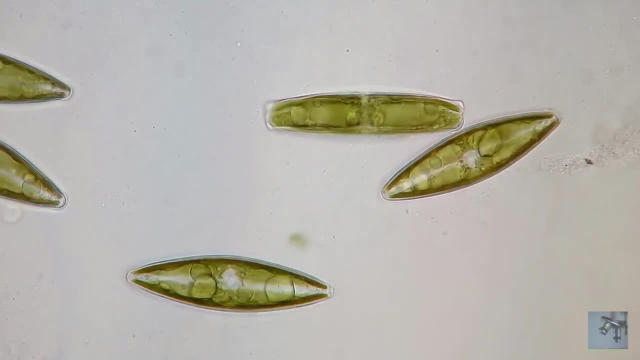 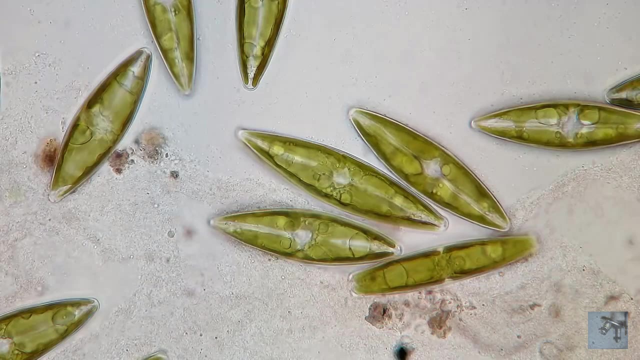 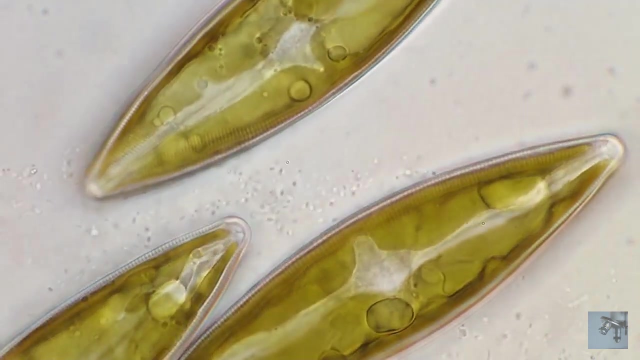 never been seen. However, a study published in 2017 in the journal PLOS1 titled Morphological and Transcriptomic Evidence for Ammonium Induction of Sexual Reproduction in Thalassiosaurus pseudonana and Other Centric Diatoms, link in description showed that the diatom Thalassiosaurus pseudonana 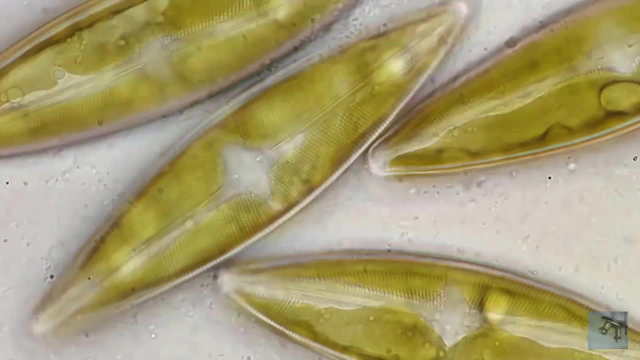 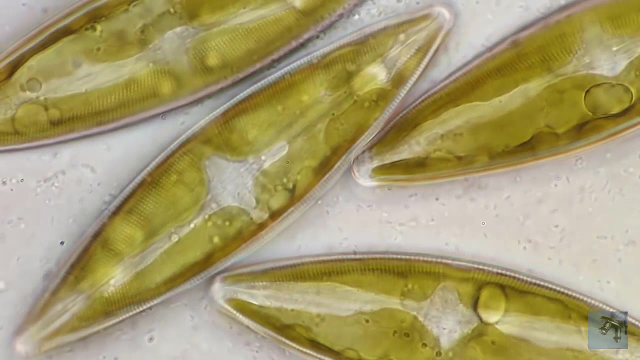 could be manipulated into changing its cell structures to be male or female. All they had to do was eliminate one of the factors that the diatom needed to grow, such as light or phosphorus, and then introduce ammonium, and the diatoms would differentiate into male and female cells. 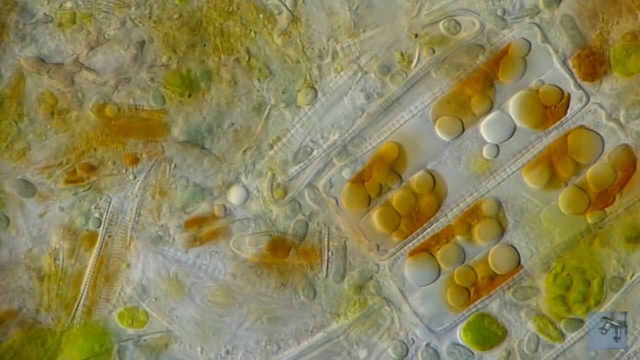 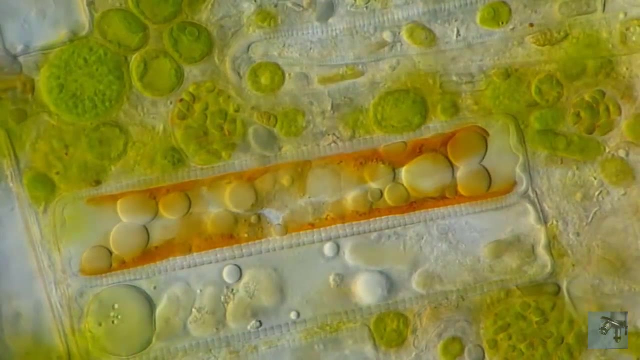 Though tiny diatoms play an important, if unseen, role in Earth's carbon cycle. they are responsible for over 40% of photosynthesis in the world's oceans and about 20% of the oxygen we breathe. Not only that, diatoms are a key source of food and energy for other tiny animals called 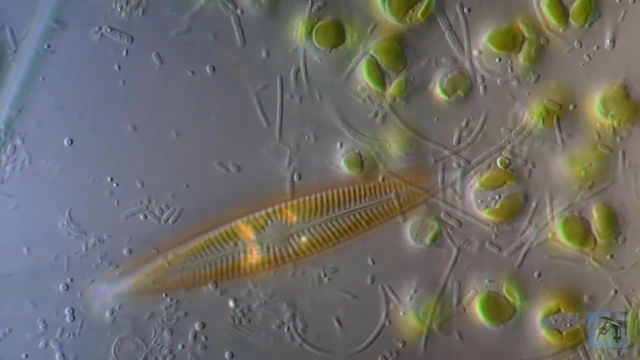 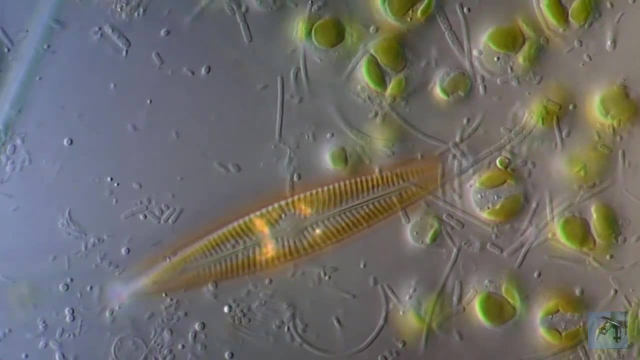 zooplankton. Zooplankton in turn sustain larger organisms like fish. so many animals in the ocean depend on diatoms, either directly or indirectly, for their survival, And without diatoms the ocean would be unable to support the amount of life that it does.